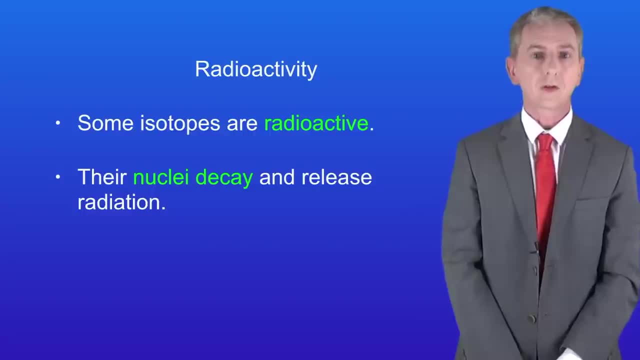 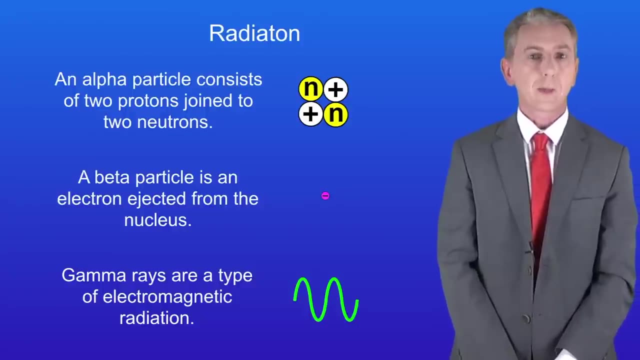 radioactive and that means that their nuclei decay and they release radiation. That's a random process, so we cannot predict when it will happen. Three types of radiation are alpha particles, beta particles and gamma radiation. In this video we're going to look at the properties. 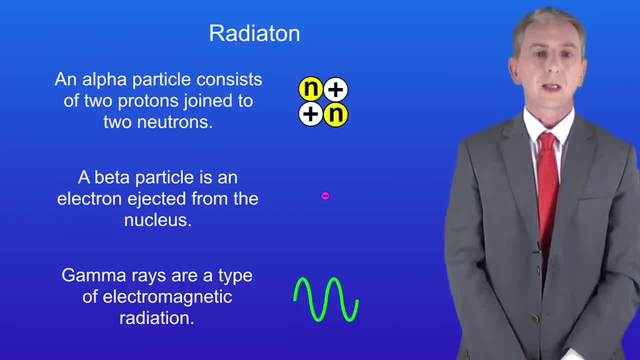 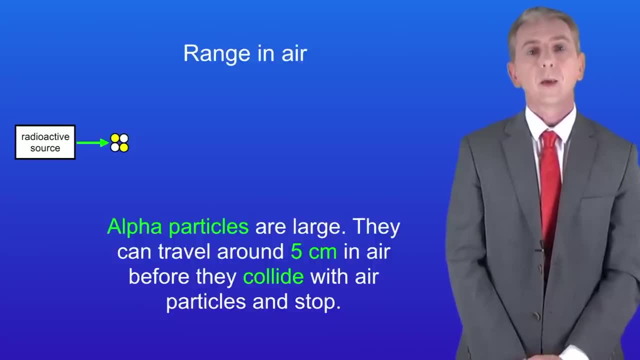 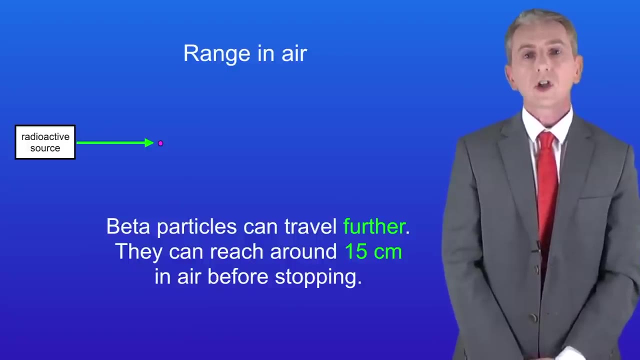 of these. so let's get started. The first key property is their range in air. Alpha particles are large. That means that they can travel around 5 centimeters in air before they collide with air particles and stop. Beta particles, on the other hand, can travel further. They can reach around. 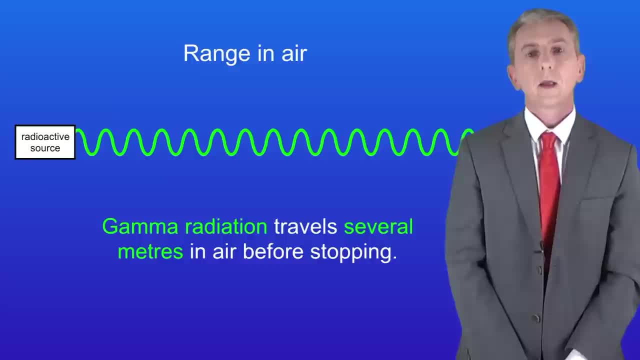 15 centimeters in air. That means that they can travel around 15 centimeters in air. That means that they can reach around 15 centimeters in air before stopping Now. gamma radiation can travel much further than either alpha or beta particles, So gamma radiation travels several meters in air. 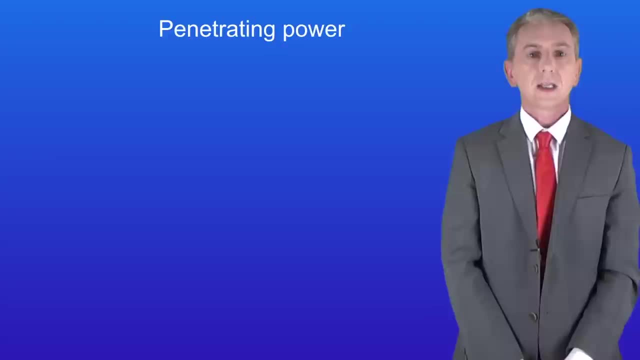 before stopping. Okay, the next key property is penetrating power, and this tells us what type of material is required to stop each form of radiation. So, starting with alpha particles, these are relatively easy to stop. In fact, alpha particles are stopped by a single sheet of paper. 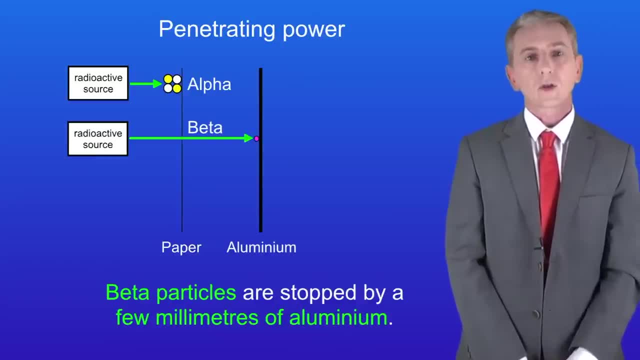 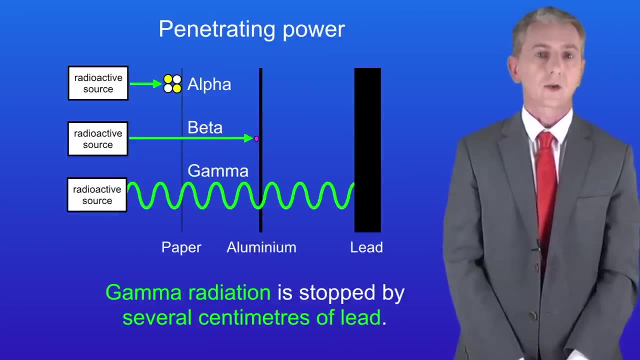 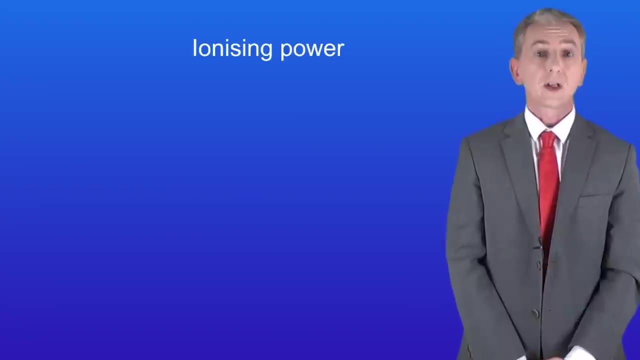 Beta particles are harder to stop. In order to stop beta particles, we need a few millimeters of aluminium. Gamma radiation is even harder to stop. So gamma radiation stopped by several centimeters of lead. Okay, the final property we need to look at is ionizing power. So first of all, we need to 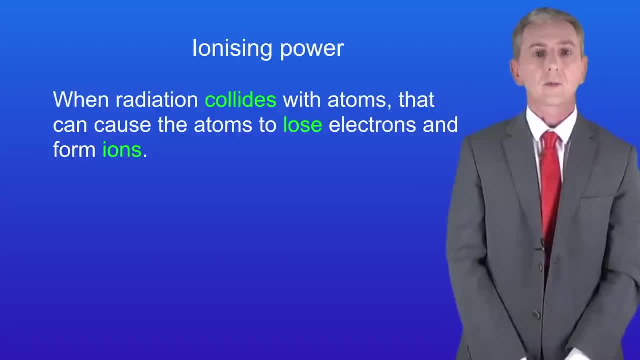 explore what that means. When radiation collides with atoms, that can cause the atoms to lose electrons and form ions, And we saw in an earlier video that the ionizing power of electrons can be that ions are atoms with a charge. Now, each type of radiation has a different. 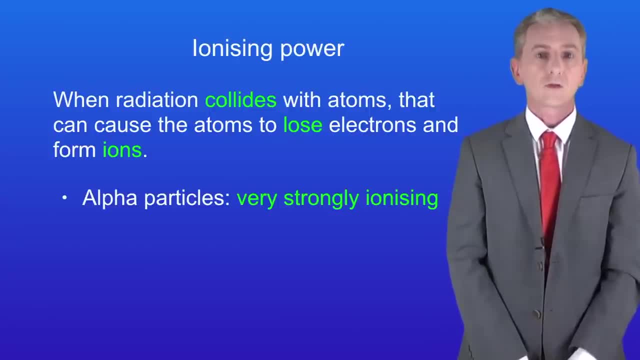 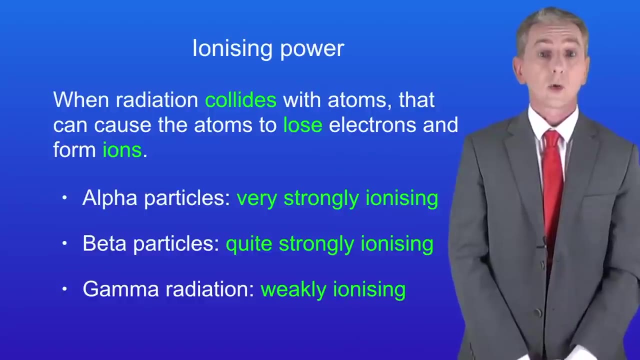 ionizing power. Alpha particles are very strongly ionizing. That means they can produce a lot of ions when they collide with the material. Beta particles are quite strongly ionizing, but not as ionizing as alpha particles. And finally, gamma radiation is only weakly ionizing. Remember, you'll find plenty of questions. 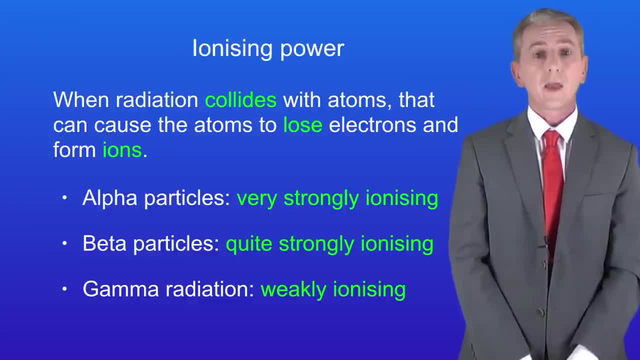 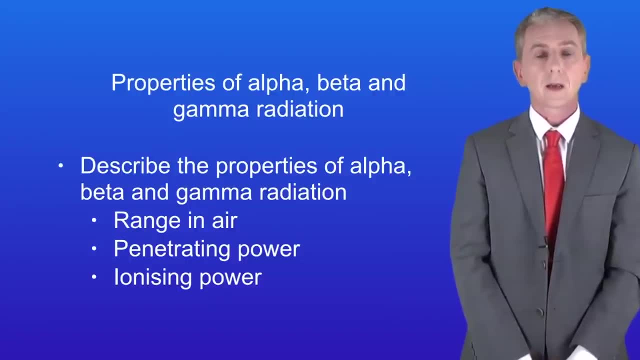 on the properties of radiation in my vision workbook, and you can get that by clicking on the link above. Okay, so hopefully now you should be able to describe the properties of alpha, beta and gamma radiation.